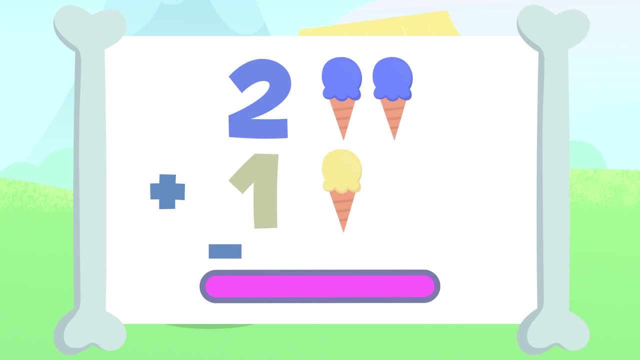 You got it. Let me try. All ice creams. together would be one, two and three Three. There are three ice creams. Two plus one equals three. We just did our first addition. The result of adding two plus one is equal to three. Well done, Dino. Let's try another. 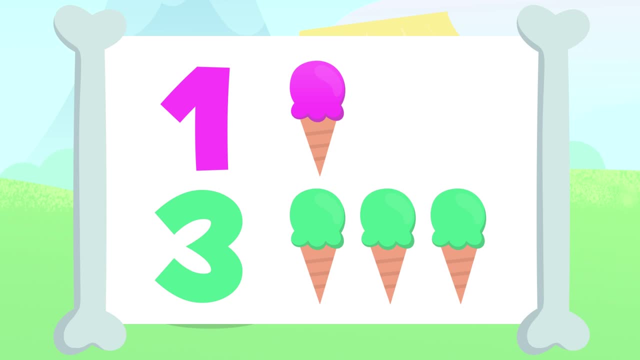 one. There's one ice cream up here and three down there. Why don't you add them up? Take your time, You got it. If we add these ice creams together, we'll have in total one, two, three and four. 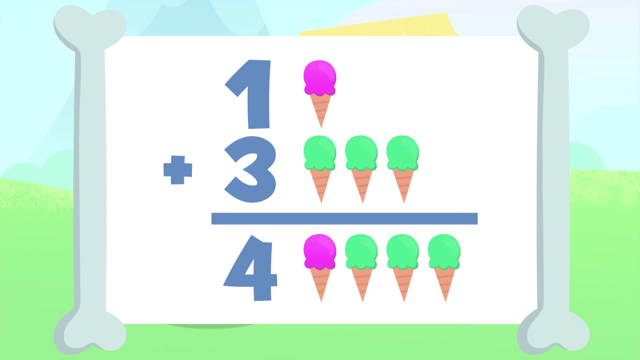 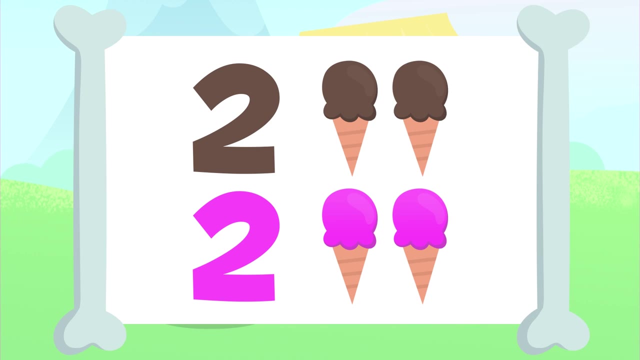 Four. We have four ice creams in total. One plus three equals four. Shall we carry on. Now you'll have to add these two. Add these two ice creams up here to those two ice creams down there. I'll give you a few seconds to add them up. 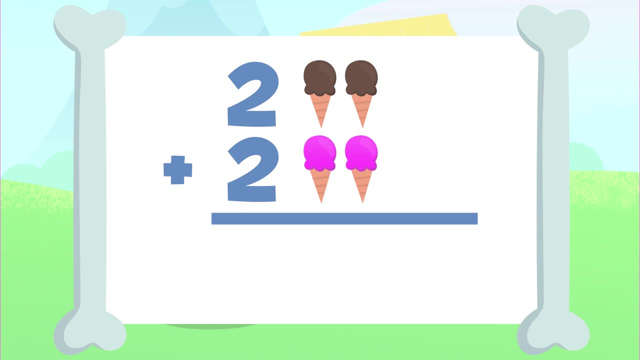 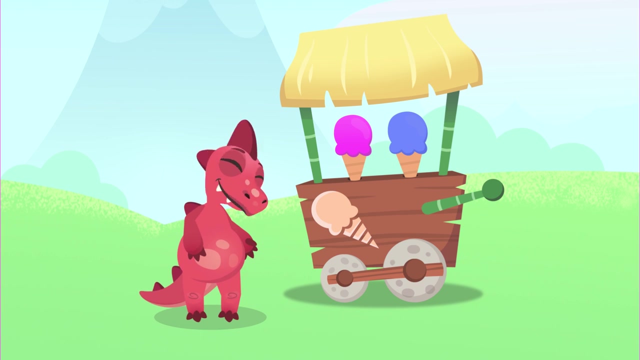 How did that go? You got it. The result of adding up two plus two is one, two, three and four, Four. There are four ice creams. Two plus two equals four. Let's try another one. You'll have to add these four ice creams up here to the one ice cream down there. 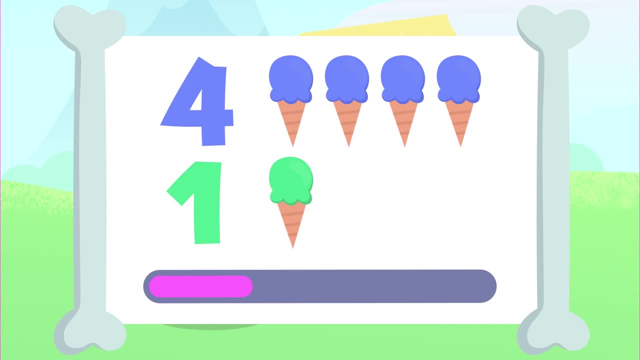 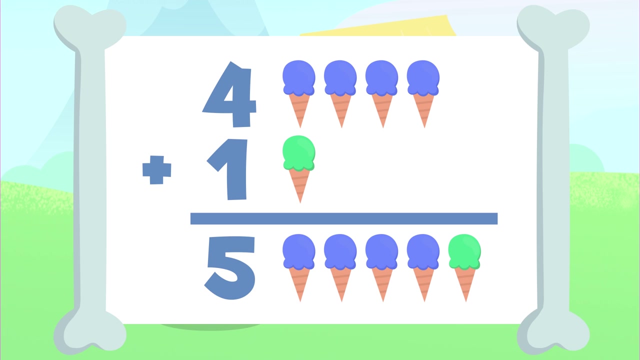 Let's go for it. You got it. The result of adding up four plus one is one, two, three, four and five, Five. There are five ice creams. Four plus one equals five. Shall we try the last one. 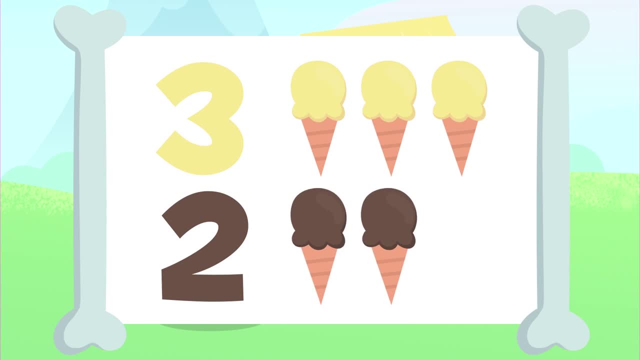 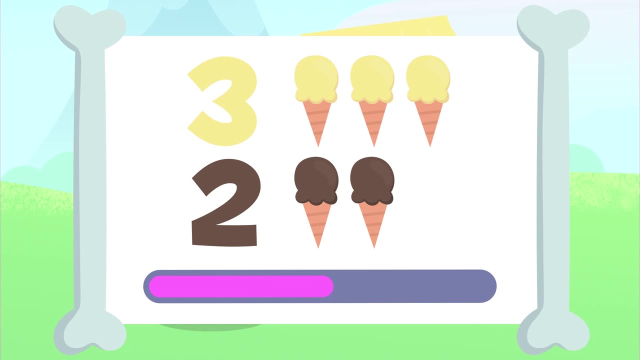 We have to add these three ice creams up here to those two ice creams down there. Let's go for it. Okay, That's it. The result of adding up three plus two is one, two, three, four and five- Five.